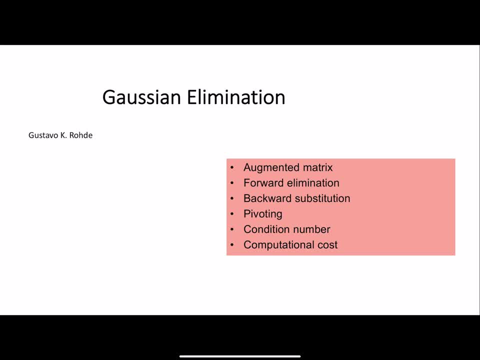 standardized and it's generic, so therefore it's easier to program To get there. to get to the understanding of this method, we're going to first define what we mean by an augmented matrix and then we're going to use this augmented matrix in the definition of the forward elimination. 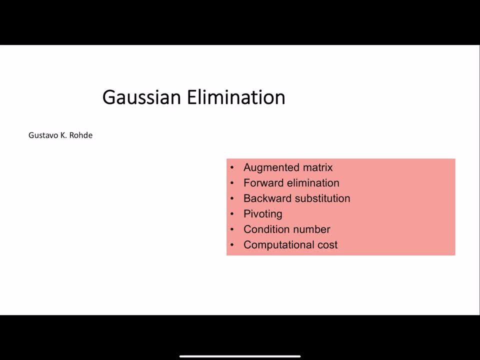 procedure, which is a way to take your linear system and rewrite it in an equivalent form so that it's easier to solve, and then it's finally solved with a method called backward substitution, Also known as plug-and-chug. sometimes We'll also talk about strategies for avoiding division. 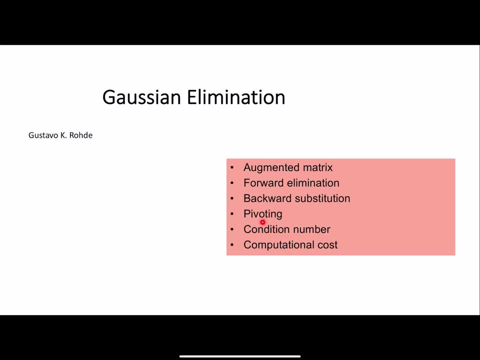 by zero throughout this process, which is also known as pivoting in this domain, We'll talk about linear systems, which are harder to solve. We'll talk about the condition number and we'll also talk about the computational cost of these procedures. So here is again our linear system. 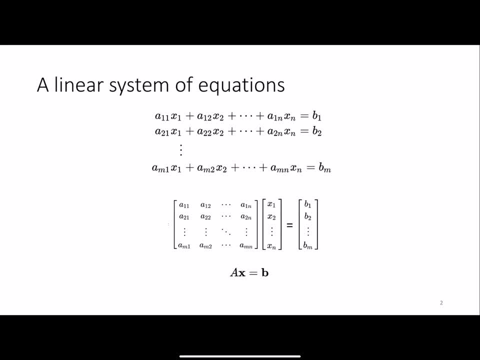 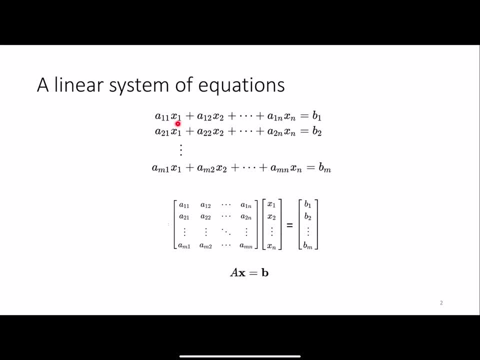 meaning there is no x squared, there is no sine of x or anything like that. rather, at most there is a number. for example, here it's denoted as a11, a12. at most there is a number that multiplies this unknowns, right. so in that sense this is a linear equation and we have a set of equations and on the 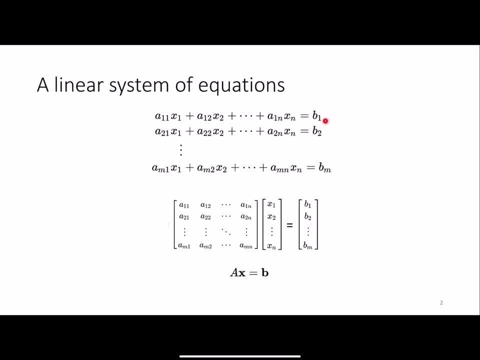 right hand side, we standardize so that there is just a number here, no unknowns, right? so we have a set of equations and, as we saw in the previous video, we can take the set of equations and rewrite it as a a matrix of known coefficients: a11, a12 and so on. a vector of unknowns equals a vector. 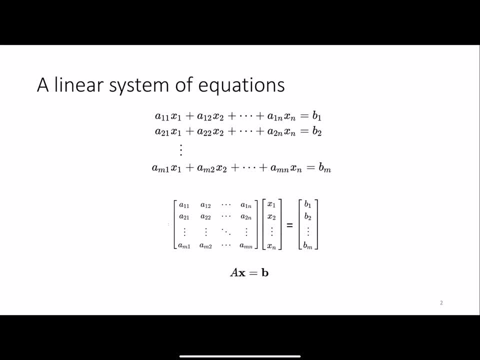 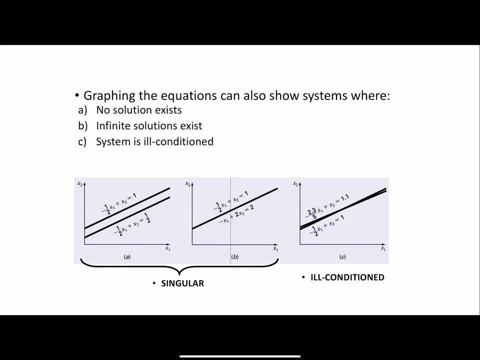 of known numbers on the other side. in other words, a times x equals b a times x, meaning matrix vector multiplication. so before we actually get into um the solution of of a linear system, we have to remind ourselves that not always a linear system has a solution. sometimes there is no solution that will exist, sometimes there. 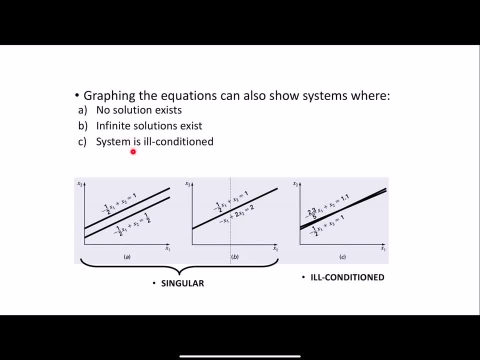 is an infinite number of solutions that exist, and sometimes this: there may be a solution that exists, but it's harder, it's hard to find. so, as we already talked about a two by two linear system of equations, in each equation, in that system, each equation can be viewed as the equation of a line. 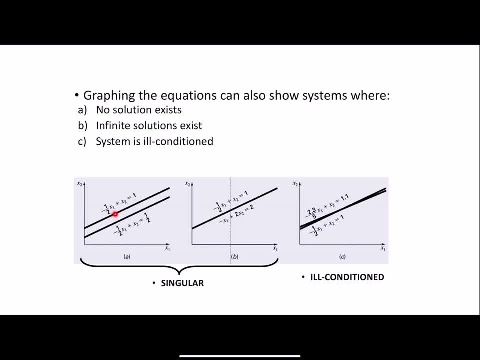 uh right, and so the linear system will have no solutions when the two equations in a two by two system imply different parallel lines. in this case there is no intersection between these two lines, so there is no point- x1 and x2- that belongs to both lines at the same time. conversely, these two lines, uh for. 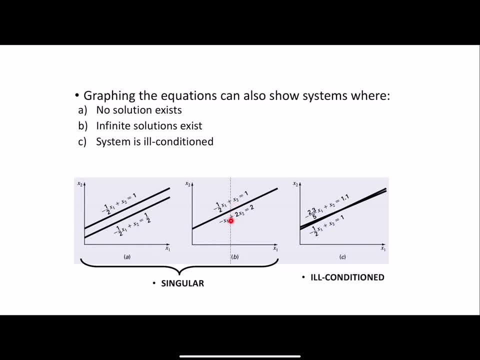 for these two equations. uh, these two equations may imply two lines which are the same line, they lie exactly on top of each other, in which case we have an infinite number of points that belong to both line 1 and line 2, so an infinite number of solutions. In both these cases, the matrix that 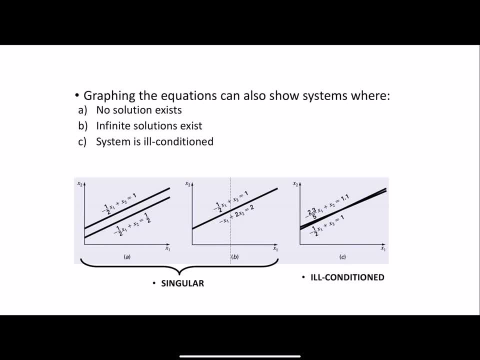 is used to represent this linear system is called singular. We can have a solution, but sometimes the solution may be hard to compute, and this is usually the case when the lines in a two-by-two system, for example, are close to being parallel, in which case a slight numerical mistake throughout. 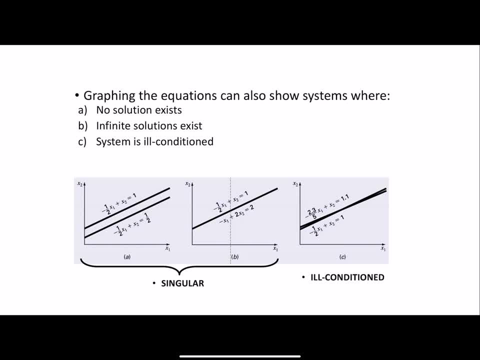 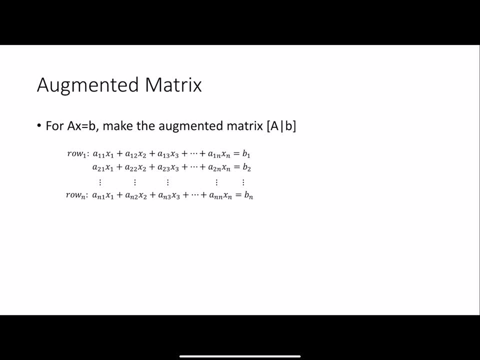 these calculations may change the answer by a large amount. In this case we call the system ill-conditioned. So with that out of the way, let's talk about this definition of what we call the augmented matrix. Again, here is our linear system and here is equation 1, or row 1,. 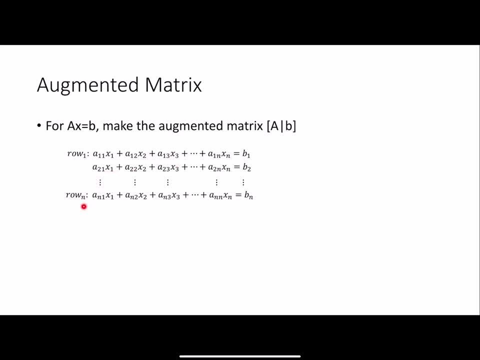 corresponds to equation 1, row 2, all the way to row n. So in this case we're looking at the square system: the same number of unknowns and the same number of equations. As we saw, it's most common to rewrite the system as a matrix times a vector of unknowns. 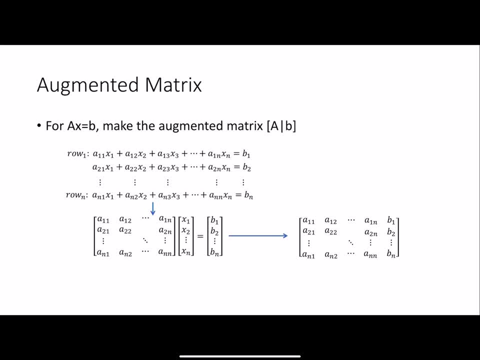 equals a vector and we're going to build what we call the augmented matrix by simply taking this vector of values b on this side and just concatenating as an extra column on this matrix a right. So here's the result: This is called the augmented matrix. 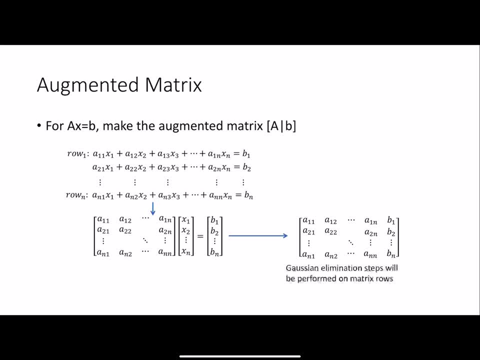 This is done so that we can do some easier bookkeeping right. We don't have to really keep the definitions of x1, x2, all the way to xn, because these are sort of implied by the problem definition. We don't have to keep writing them. 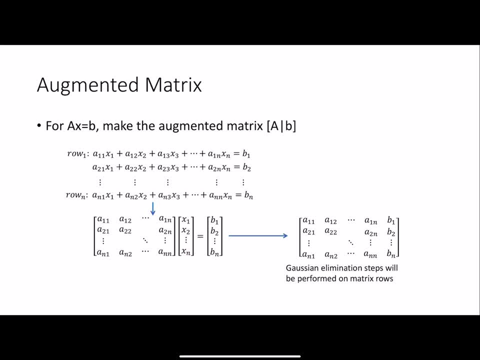 right. We know there will be n unknowns in an n by n system, And so what we're going to do now is define operations that are going to be performed equation by equation or row by row in this augmented matrix, in such a way that we can get the answer to the question. 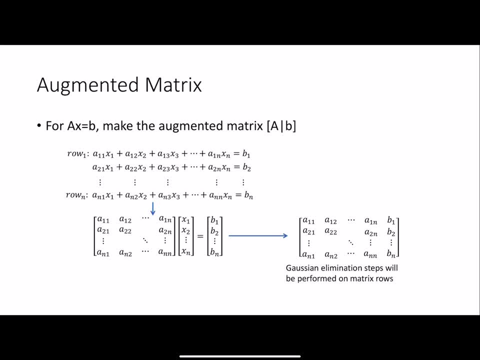 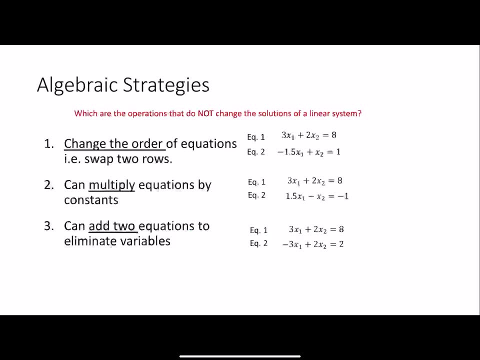 a s 2, simplify it so that we can use a simple algorithm to backward substitute and find the actual value of the unknowns. How are we going to do this? We're going to take advantage of a few basic- I would argue- commonsensical- rules about what we can do to an equation. 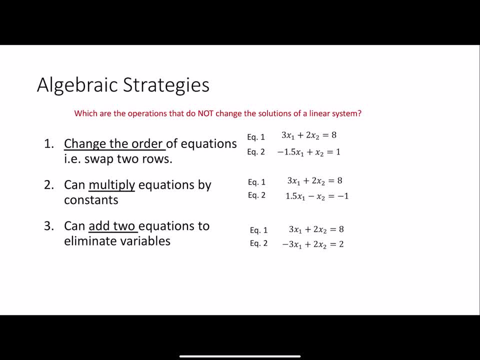 without changing the solution of the system of equations, Right? First thing to note, let's say we have a two by two system of equations, So we're going to do the same thing. right, We're going to do the same thing, but we're going to do it in a different way than what. 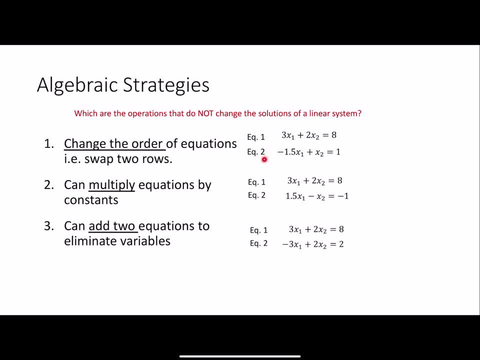 we did before. So we're going to do this in a different way than what we did before. So Here is equation 1 and here is equation 2.. It doesn't matter as far as the solution is concerned if we write equation 1 first and equation 2, or we switch the order. 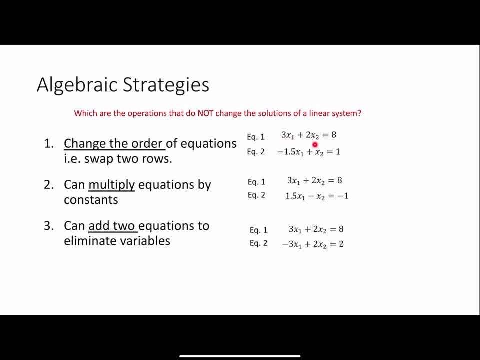 It doesn't matter, because the x1 and x2 that satisfy both equations at the same time will be the same as the original system. So we are allowed to switch the order, essentially swap two rows of the augmented matrix. Likewise, we can take any equation, either equation 1 or equation 2, and multiply it by some number that we would like to multiply it by. 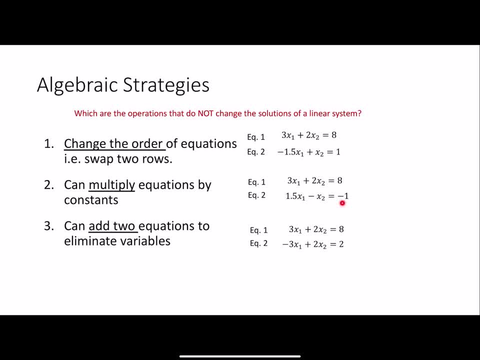 For example, we can take equation 2 here and multiply it by 2 and replace equation 2 by the same equation multiplied by 2.. The same thing that I said for the change of order applies here. The solution, that is, the value of x1 and x2 that satisfies both equations at the same time, will not change. 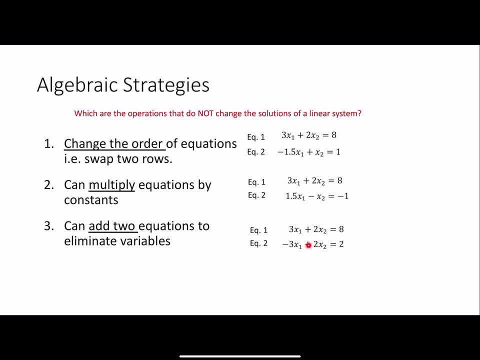 Finally, We can add two equations in a linear system and replace one of these equations by this addition. And the same can be said here that the solution- x1 and x2, will not change based on this addition. So here is an overview of Gaussian elimination. 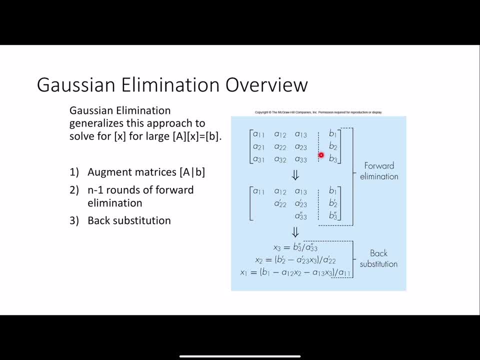 So here is our augmented matrix. We've taken a 3x3 system of equations. Again, we removed the unknowns, Because those are implied, And we concatenated the b vector on the other side. So now we have this array, essentially. 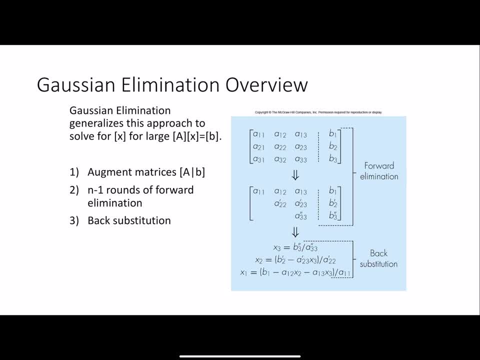 The first step in Gaussian elimination is to use the operations we just talked about: Multiplying the line by the same factor, Adding the same number to both sides of the equation, and so on. We can use these tricks to rewrite this system of equations into another system of equations. 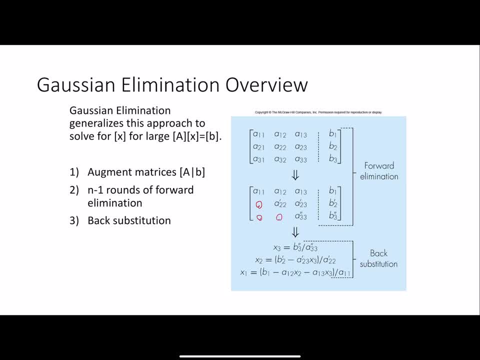 Where the values below the diagonal will be zero. So the solution to this system equation and the solution to this system of equations again are the same, So we can solve either. This one is easier to solve, for example, because the value of the unknown x3 will just be given by b3, 2 prime divided by a33, 2 prime. 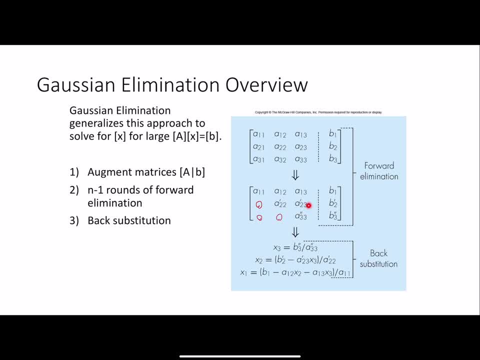 Once we know the value of x3. We plug it in here and then we find the value of x2, very simply, We take this term, subtract it to the other side and solve for x2.. Likewise, we know x2 and x3, in this case, we plug it up here and we solve for x1. 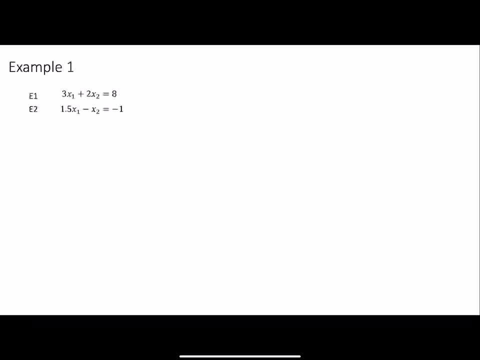 So this is known as backward substitution. So let's look at a quick example of how to do this forward elimination procedure. We have here a system of equations: Equation 1. And equation 2.. Right, And so we're going to now leave equation 1 as is. 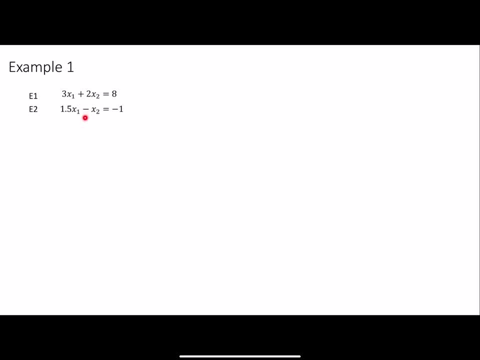 And we're going to modify equation 2 so that the first term here will be zero Right. And again we're going to modify by either multiplying both sides of the equation by the same number or adding the same number to both sides of this equation 2.. 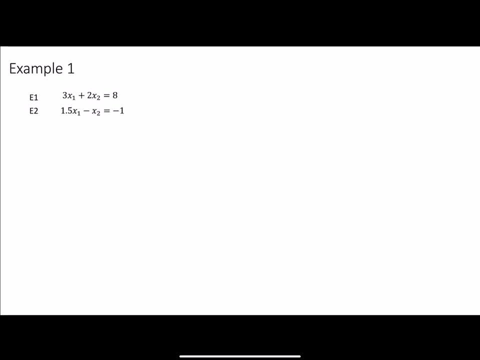 So here's one trick. Let's take a. Let's Let's take equation 2 and replace it by equation 1 minus 2 times equation 2.. So let's do this Right. So let's write equation 1 here on top. 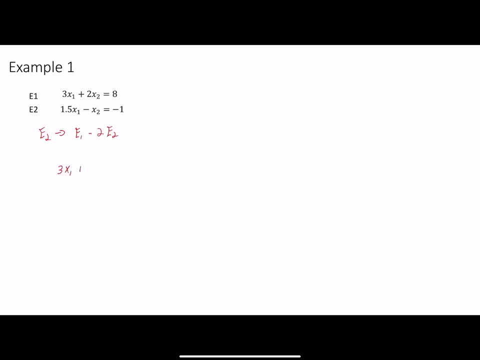 That's going to be: 3x1 plus 2x2 equals 8.. And now let's write here At the bottom 2 times. So here's equation 1 again, And here's equation 2.. So Sorry. 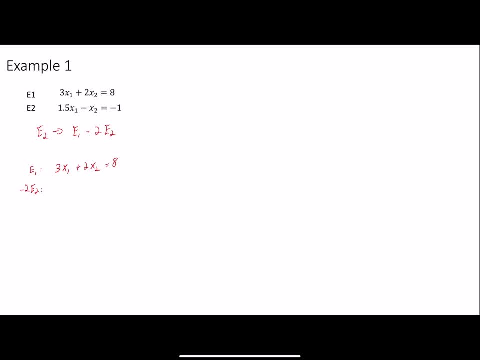 This is going to be minus 2, equation 2.. Right, So this is going to be minus 3x1.. Minus with a minus becomes a plus, So that is going to be plus 2x2.. And of course, we have to do the same thing to the right-hand side of equation 2.. 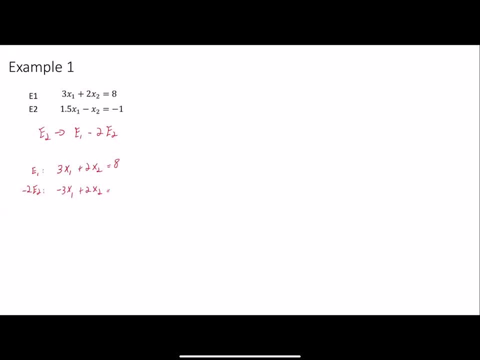 Over here, So that's going to be minus 2.. Minus becomes a minus, So that's going to be 2.. Right, And again we're going to add these two terms, as we just stated over here, And so this result will be 0x1.. 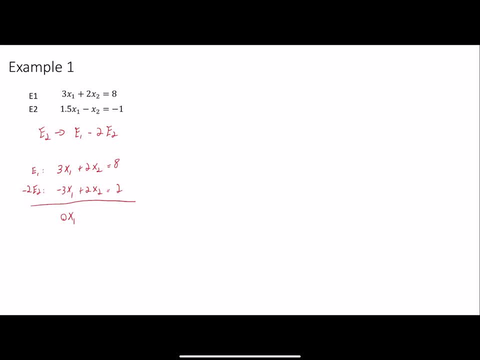 Right, Minus 3 with 3 becomes 0. This is going to be plus 4x2.. And this is going to be 10.. Right, So We're going to now take this result and replace equation 2 by that. 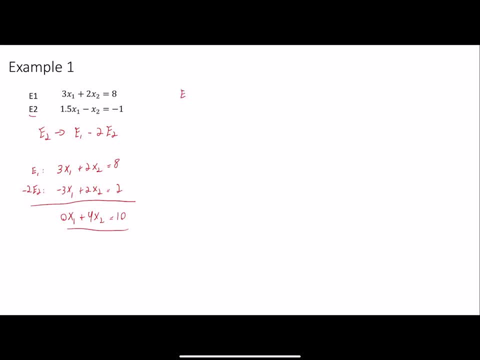 So let's rewrite our linear system. So this is going to be: equation 1 will remain the same as we had before: 3x1 plus 2x2 equals 8.. And now the modified equation 2, which we call equation 2,, let's say prime. 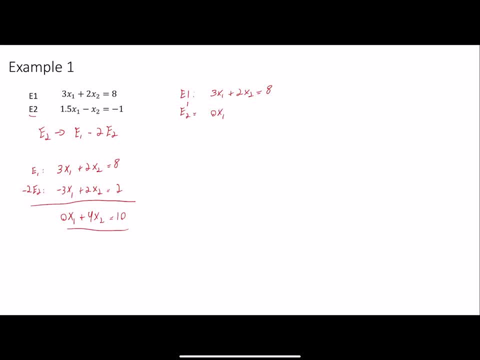 Right Will be 0x1.. Plus 4x2 equals 10.. And in this case we're done. We have performed forward elimination Because, as you can see, now we take this matrix out, So we rewrite this in standard form. 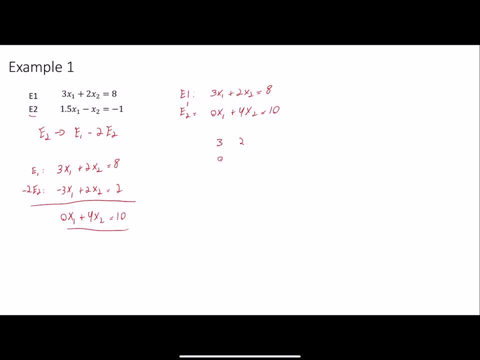 We have 3,, 2,, 0,, 4.. And of course we're going to add our extended matrix, augmented matrix, here. So here's our thing And you can see, For this part of the system, the numbers below the diagonal are 0,. 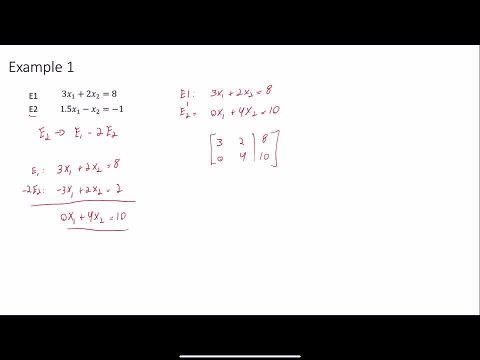 which is what we said we wanted to do In this case. we accomplished it. So now we can apply the method of backward substitution Right. So from equation 2, prime, here we can now solve for x2, because there was a 0 there. 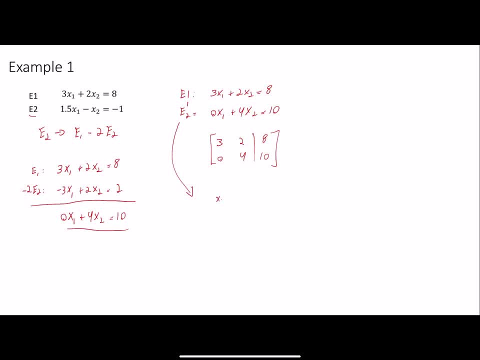 So there's only one unknown variable there. So x2 here will be equals to 10 divided by 4.. And now, once we know x2, right, we plug it into equation 1 over here, And now we have 3x1 plus 2 times 10 divided by 4.. 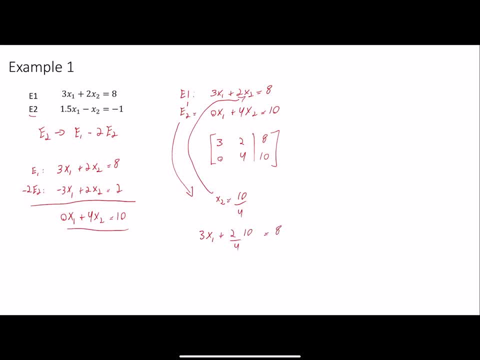 And that has to be equal to 8.. Right, So once we have this here now, of course we can just move this to the other side and divide the whole thing by 3 and we have our solution. So we can do the same thing with a 3x3 system. 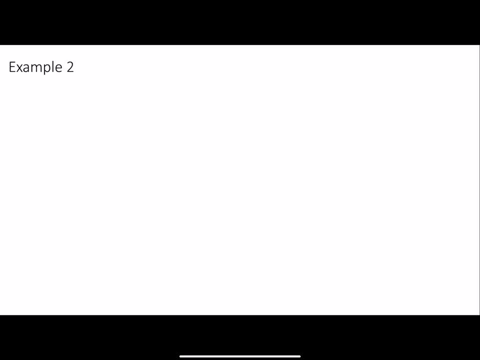 Right. So let's rewrite an equation here for a 3x3 system. So let's say x minus 3y minus 2z will be equal to 6. And let's say this is equation 1.. Equation 2 will be equal to 2x. 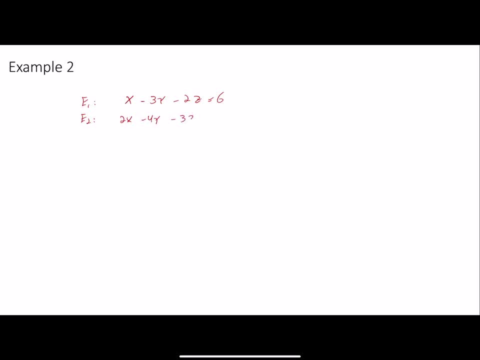 Minus 4y minus 3z equals to 8.. And equation 3 will be equal to minus 3x plus 6y plus 8z, equal to minus 5.. So let's take a look at how to solve the linear system. 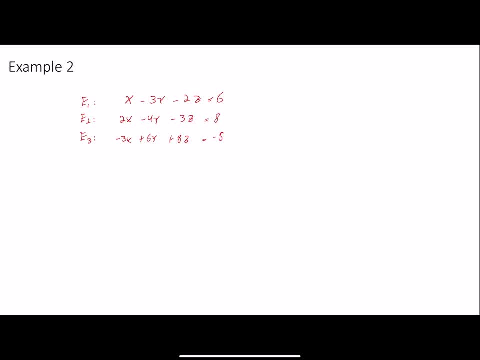 Right, So let's apply the forward elimination procedure here in this case. So step 1, we're going to now work on equation 2.. Right, So we're going to leave the strategies, to leave equation 1 the same, And now we're going to work on equation 2. 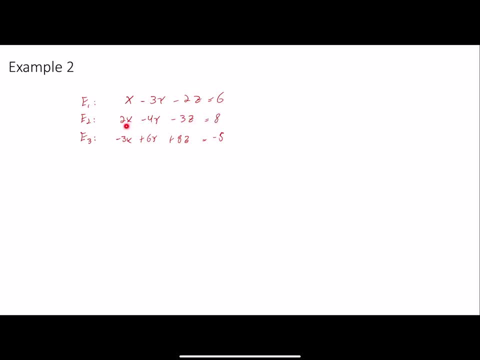 and try to eliminate equation 2 and 3.. And we're going to try to eliminate the value of this value, We're going to try to set to 0. And this also, we're going to try to set to 0.. Right. 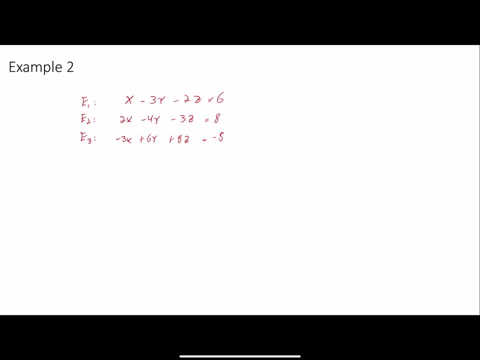 So here is one idea. I mean, there is There's no unique solution here. In fact, oftentimes there are many ways to do this. But one way to do this we can do is we can take equation 2 and replace it by minus 2 equation 1. 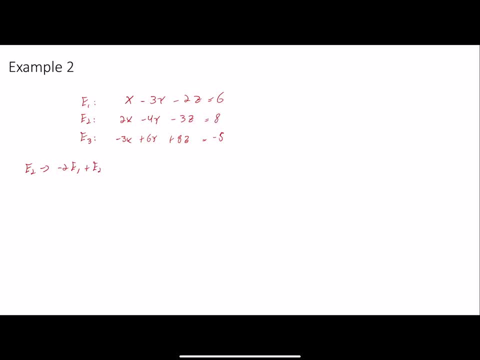 plus equation 2.. Right, And for equation 3, we can Replace it by 3 times equation 1 plus equation 3.. So if you follow the same procedure that we just did in the previous example and you substitute, now you have a new system. 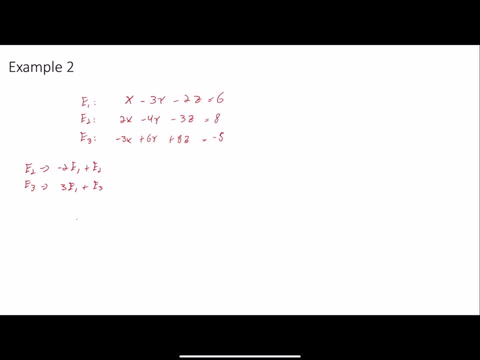 which we'll call Again. equation 1 remains the same, Right. So we'll have x minus 2.. 3y minus 2z equals 6.. Equation 2 prime. now I write equation 2 prime to make sure that. 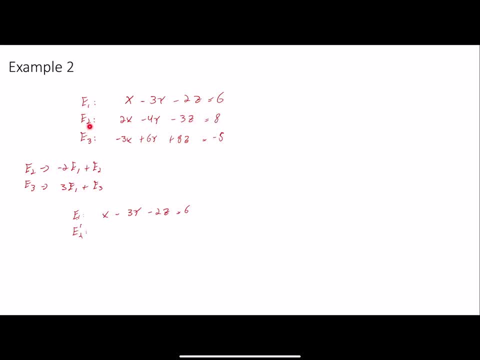 we understand this is a different equation than equation 2.. Right, So this is going to be. If we perform this operation here, we substitute the original equation 2 by this modified version. So this is going to be 2y plus z. 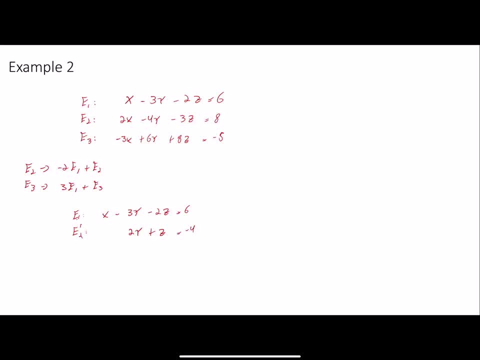 equals minus 4.. And equation 3- prime again, because we replaced the original equation 3, is going to be minus 3y plus 2z, equal 13.. So our original system was here, And now we have rewritten it over here. 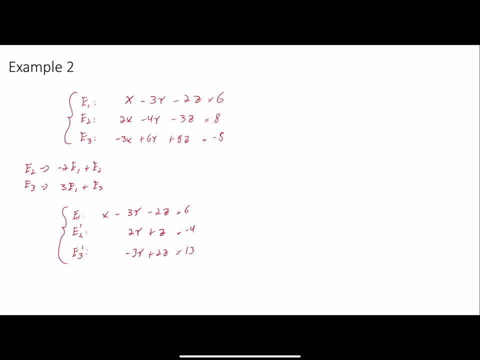 The solution of That is, the points x, y and z that satisfies all these three equations should be exactly the same as the x, y, z that satisfies these three equations. So the solution hasn't changed. But you can see that we have rewritten the system a little bit. 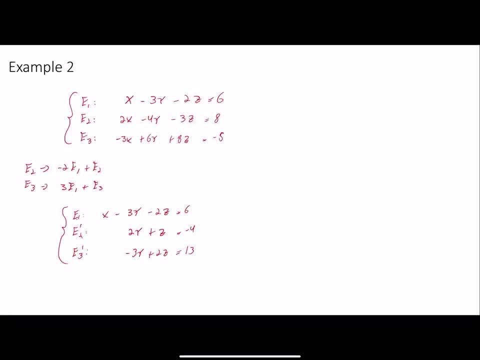 Now we have done right. We have set these variables here to be 0x, 0x, Right. So that's what we have to do now is work on this particular variable. Let's set that to 0 as well, by performing these legal operations. 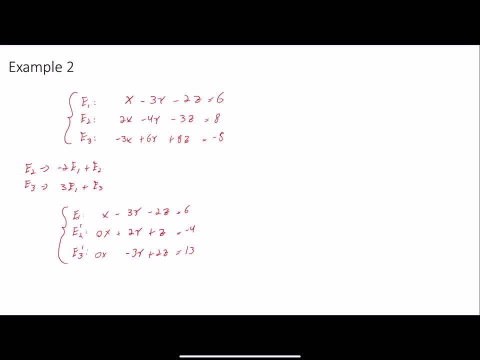 So let's replace equation 3, say, with 3, equation 2, plus 2, equation 3.. Right, So if we do this we're going to end up with a new system now, So in the last. So the first two equations won't change anymore, right. 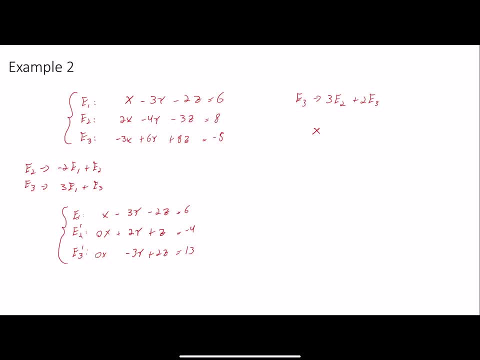 We already worked on them, So the equation number 1 is still x minus 3y minus 2z, equals 6.. Equation 2 will remain as before, So it's going to be 2y plus z equals minus 4.. 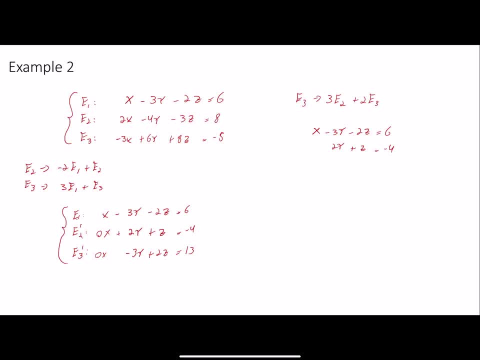 And now equation 3,, as you will see, will become 7z equals 14.. So here's our third version of the system, And from here we can see that z is equal to 14 divided by 7. Right. 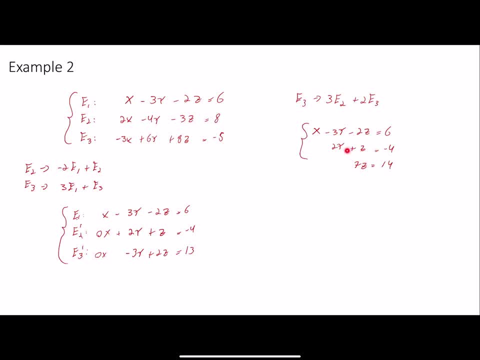 Once we obtain z, we plug it in here and then we can solve for y. Once we have y and z, we plug both numbers here and we solve for x, And that will be the business of backward substitution. So how do we write this? 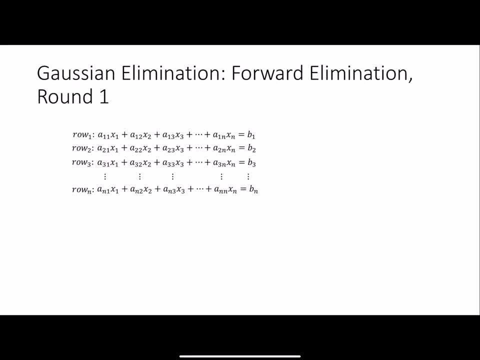 in a more standardized form for a generic linear system, right? What is the general strategy to follow here? So you work on rows of this matrix, one row at a time. So, for example, you start and you leave row 1 or equation 1 unchanged. 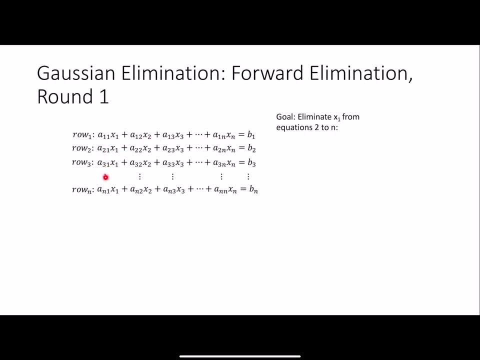 And you work to zero out all the elements of a21, a31, and so on, all the way to n1, n1, below the first pivot point, Right. So what does that mean? Equation 2 or row 2. 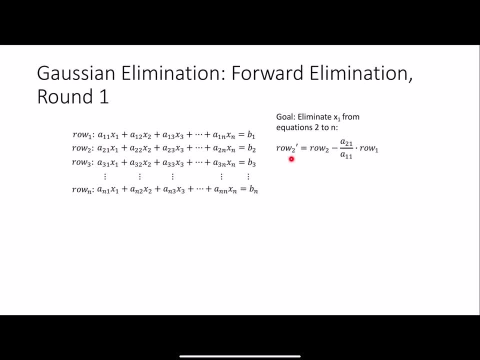 now will become equation 2 prime or row 2 prime, And you will note that all you have to do is subtract a21 divided by a11.. So a11 is our pivot division point times equation 1.. If you perform this operation here, 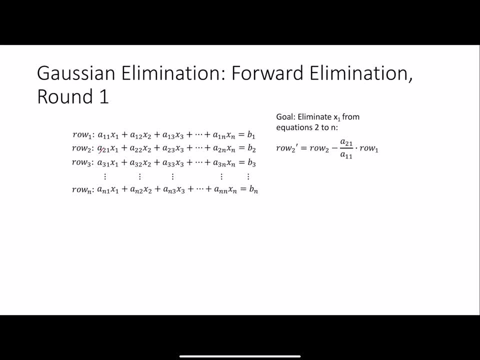 what will happen is this guy in the new version of the equation will become zero. Of course you do the same for row 3, row 4, and so on. right? So all you keep the same division point a11,. 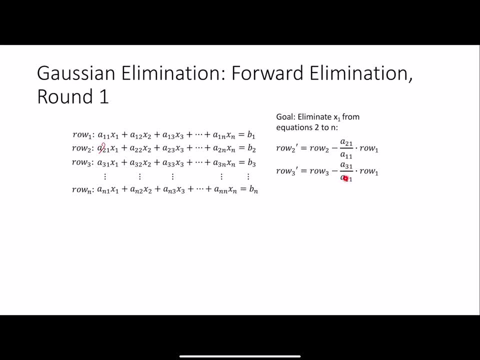 and you divide, you know, a31 by that, by that, by that number. But otherwise, you know, all that's changing is that from row 2 here becomes row 3 or equation 3.. Right, You can see. and this: 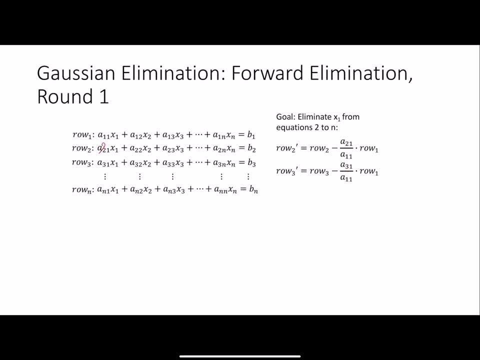 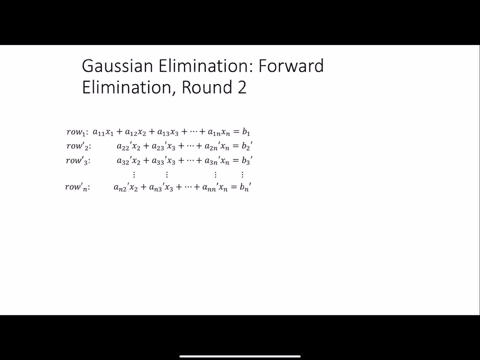 the coefficient here also changes. But you can see how this is easier to program Right And you repeat the entire process for all of these numbers, And that's step 1.. Now for step 2, now you have replaced each of these equations here. 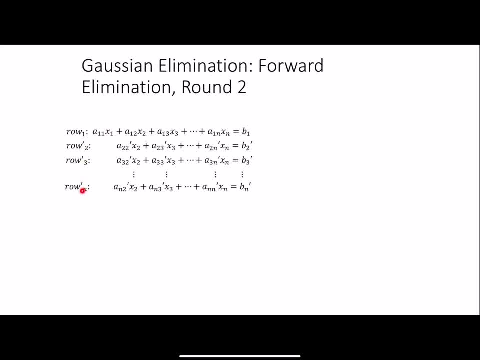 by the prime versions, Right? So now all of these elements here have become zero. Now you do the same thing for these guys here, right? You leave a22 as the pivot point, but you apply all of the same ones from there. 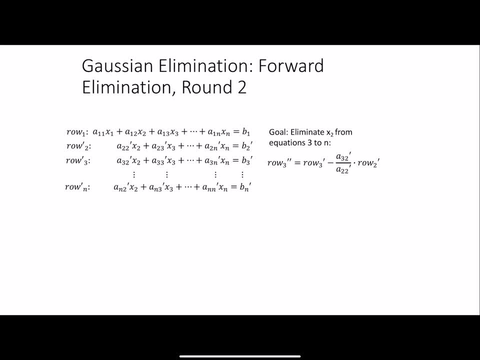 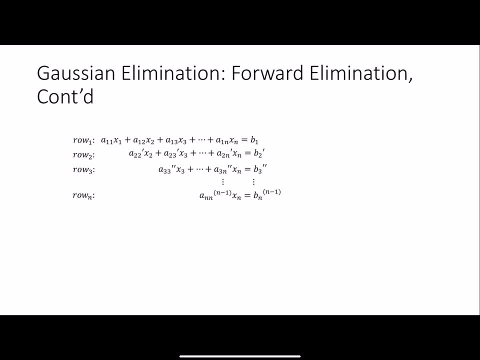 And the procedure is identical, right, But instead now we're playing with this value, this value and so on, And you keep doing this all the way until the very bottom, or you do it n minus 1 times, right? 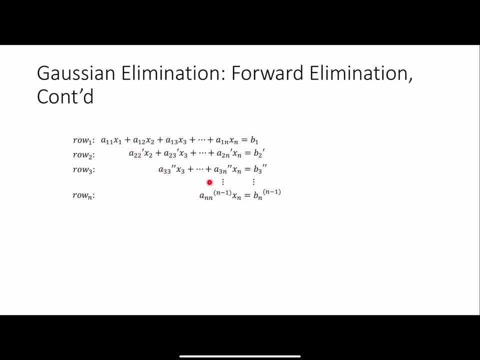 Because you'd skip the first one. So you have one times less than the size of the system, But by the time you repeat this enough to get to the bottom. you end up with a very simple equation here And all you have to do to get the last value of your unknowns. 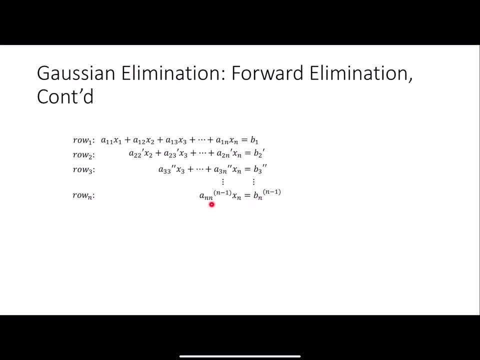 is divide bn minus 1 here by a and n to the n minus 1, right, And that's the general procedure for what's called Gaussian, the forward elimination part of the Gaussian solution to linear system of equations. Now, once you have performed this part, 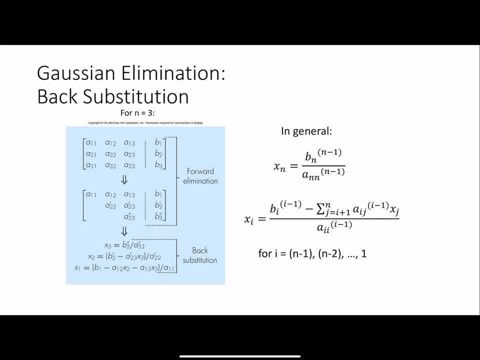 you perform the backward substitution, which in this case we already talked about, right We? we simplify the linear system to be 0 below the diagonal, so we can get x3 to be simply b3: 2 primes divided by a33 prime right. 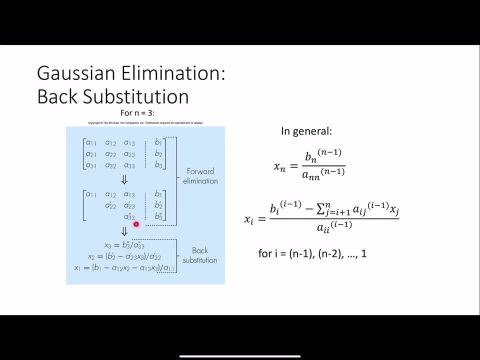 So this is what we're saying over here, this part of the formula, And then once we have x3, we plug it in here and then we only have to solve for x2, right, And here is the solution of for that formula, where the sigma here is summation, right. 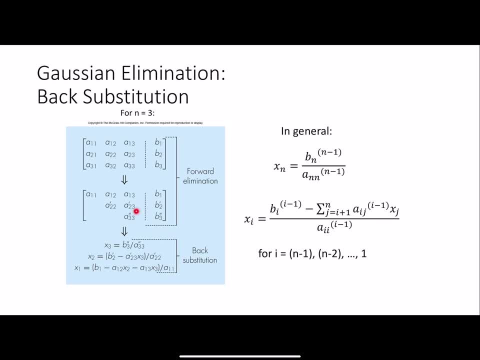 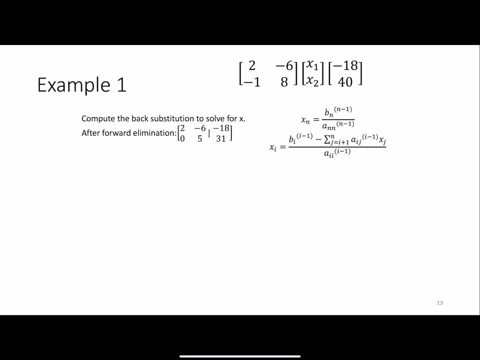 And you repeat all the way back, uh, to the system, all the way until you solve back for x1.. So this is what's called the back substitution. All right, so let's perform this back substitution here, For example, in this case: 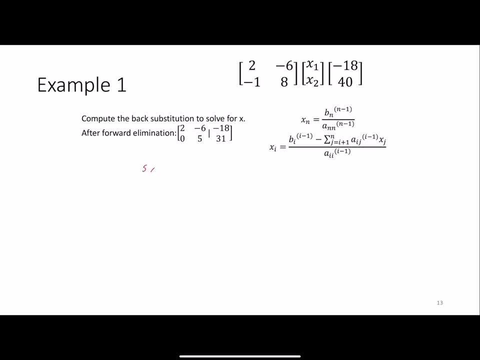 we have that 5x2 will be 31,. right? Where did I get this from? I got this from the bottom line of this augmented matrix, And so I perform this formula here. So x2 will be 31 over 5, whatever number that is. 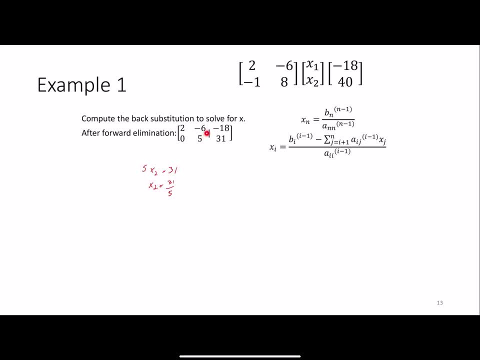 Now I take this number here and I plug it in up there, right? So now our new equation will be: 2 minus 6 times 31 over 5 equals to minus 18.. Right, Sorry, this should have been. let me find an eraser. 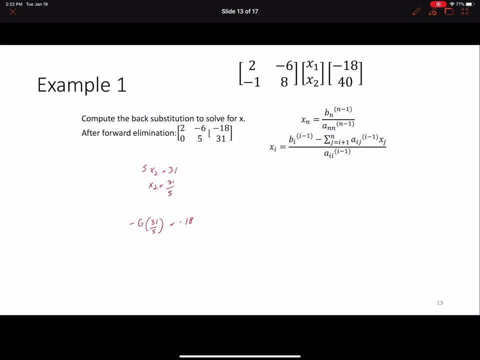 This should have been 2x1, right? So this is going to be 2x1, right? So that's more like it. So now we take this number here and put it on this side and then divide by the coefficient right. 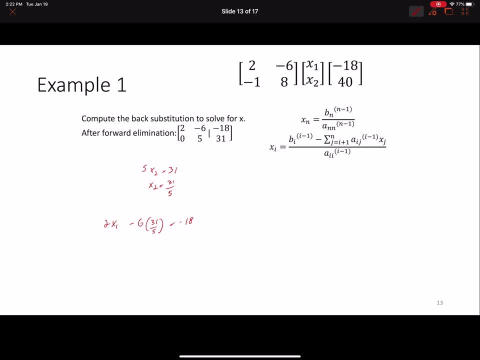 So this is exactly what this formula is saying here. So let's do that. So this is: x1 will be minus 18 plus 6 times 31 over 5 divided by 2, which is this formula here. So here is, you know, the summary of this procedure. 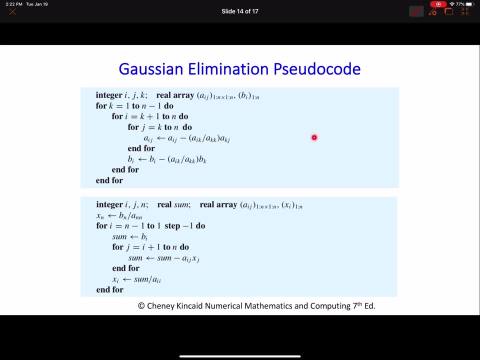 There are two parts: the forward elimination procedure and then the backward right. So The first part you iterate. you know you do this n minus 1 times right? So here you're going to rewrite those equations and you're going to substitute each number in that augmented matrix. 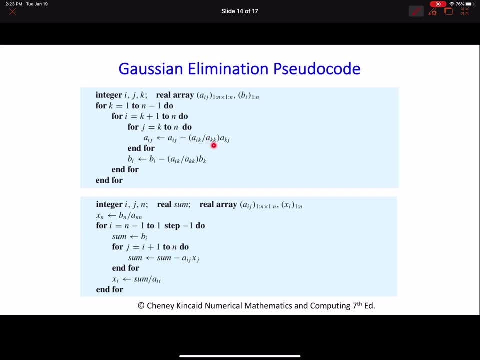 by this number instead, as we just talked about right. And of course, you do the same thing for the right-hand side, And this procedure will give you a new augmented matrix, but one that has been where the, the values below the diagonal, have been set to zero. 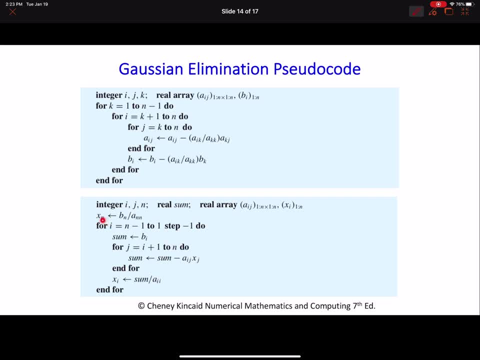 You then start the backward substitution by assigning the value of the last unknown right. That was easy. And then you substitute. First you compute the sum right. You start with the sum as set over here and you keep adding to the sum this negative value right. 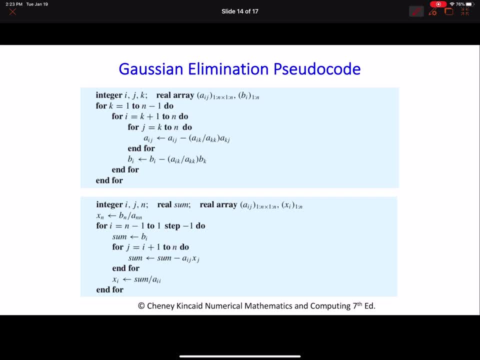 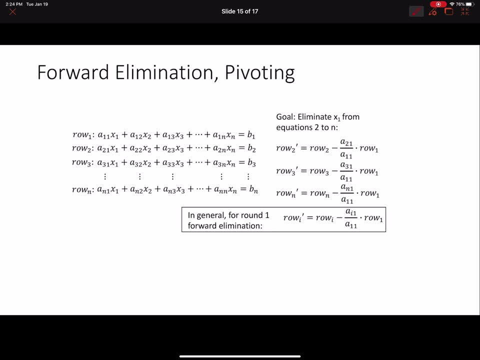 And at the end you just divide the sum by the right pivot and then you got the solution for that particular value. So one issue can come up here, right, And the issue is here: what if the pivot in this case is a11, right? 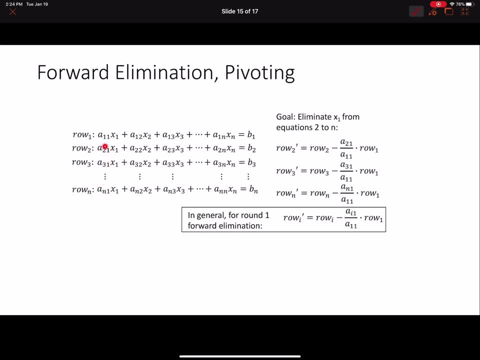 So we're looking at zeroing out all these elements. so we take the a11 as the pivot. What if this guy here was zero or even close to zero, right, But if it was strictly zero, you have a21 divided by zero. 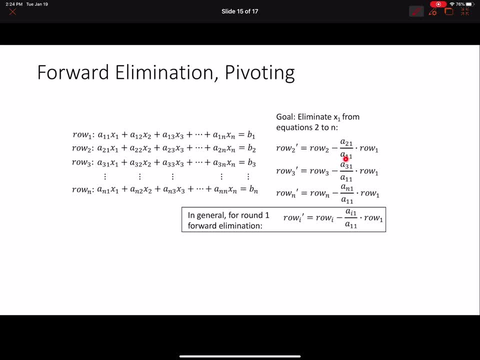 What sense does that make? Like none. So we can't have division by zero. If we do have division by zero, the whole procedure will fail. So what can we do? Here is where that first rule we talked about about. what can we do to this linear system that 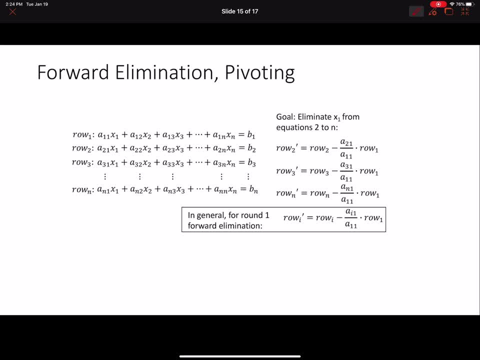 doesn't change. the solution is reverse the order. right, So I can, If this pivot point here, which in this first row is a11,, if this is zero first, what I can do is I can, I can search and look at the other equations. 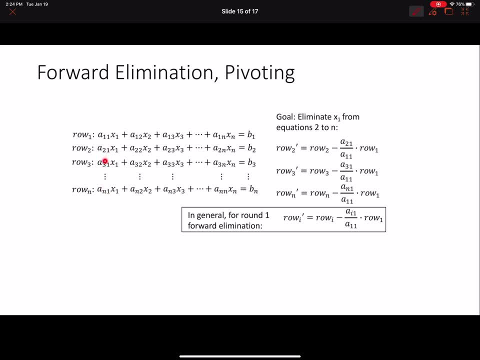 Is there any other equation where the front number here is not zero, And if so, I can just put that equation to be the first one instead and solve this rearranged system instead. right, This will avoid us dividing by zero and may still allow us to find a solution to the linear system. 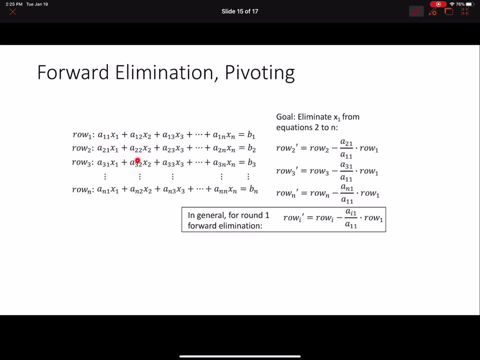 Of course I don't do that just for the a11 procedure. When I'm zeroing the values below a22, for example, I do the same thing. I look below and see if a22 is zero. I look below and see if there is one that is not zero. 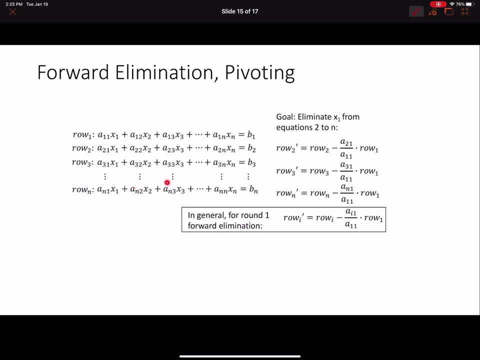 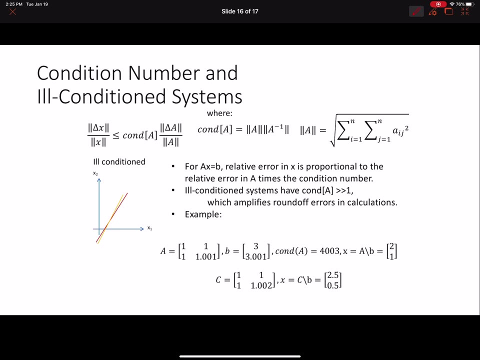 and I modify that system. right. You can do this for any pivot point. This is known as pivoting. It's a good thing to do to avoid issues with division by zero. As we talked about at the beginning of the video, there are some systems that may have a solution, a unique solution, but they may be hard to 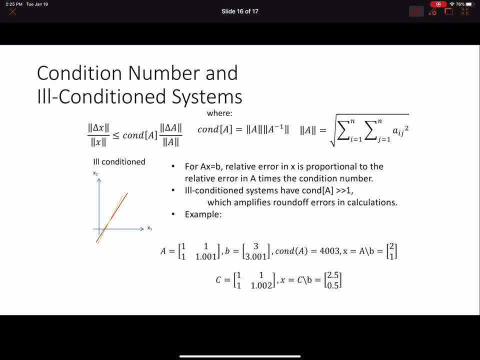 to find, numerically difficult to compute, and one, one number, one gauge that we can use to see how difficult a system, a linear system, is to solve is the so called condition number, and the condition number is defined as the matrix norm in the multiplication of the mid to matrix norms. the original system. 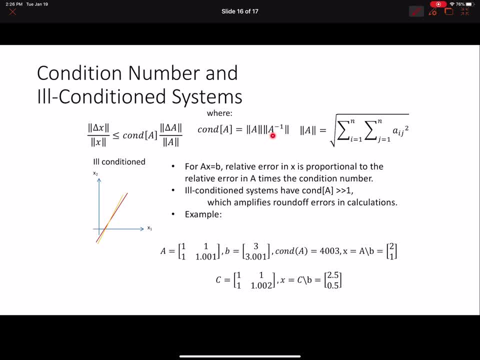 the original matrix describe the linear system as well as the inverse of the matrix. this norm multiplied together is known as the condition number. systems that are difficult to solve, where the lines are close to being parallel, have condition numbers. they're very much, much larger than one and they indicate again. 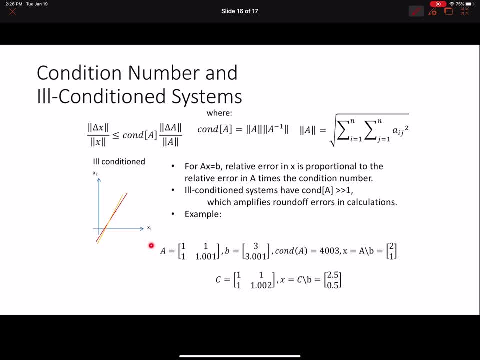 that these lines are close to being parallel. so here is a particular example, right? so let's say we have this linear system here. where the a matrix is is this one and the B matrix is that the condition number is four thousand and three, the actual, the real solution to the system.